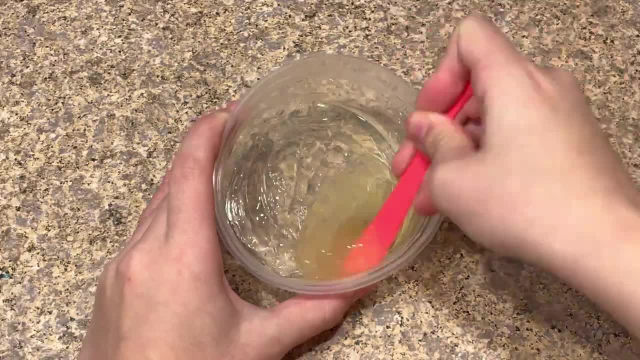 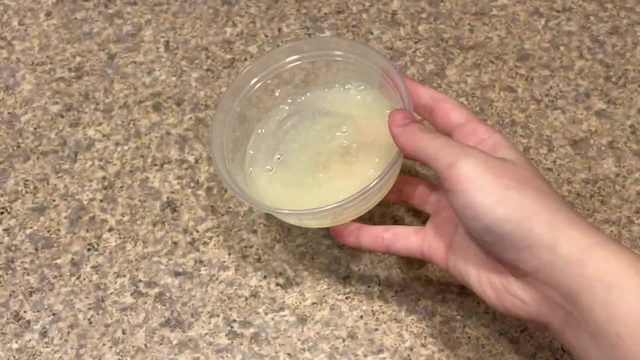 going to do that now. That looks like just enough mixing. It got super, super bubbly, as you can see, And this is what thickens up the soap to make actual no-glue slime. And now I'm going to get my toilet paper out. 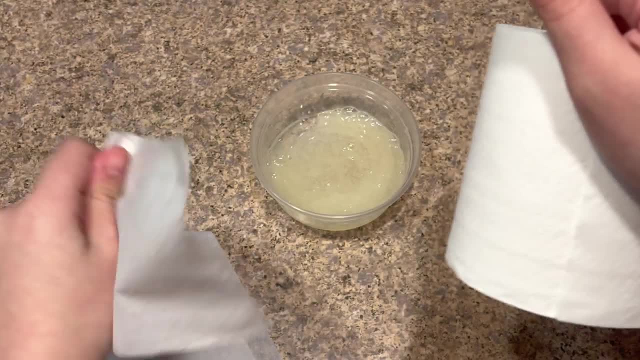 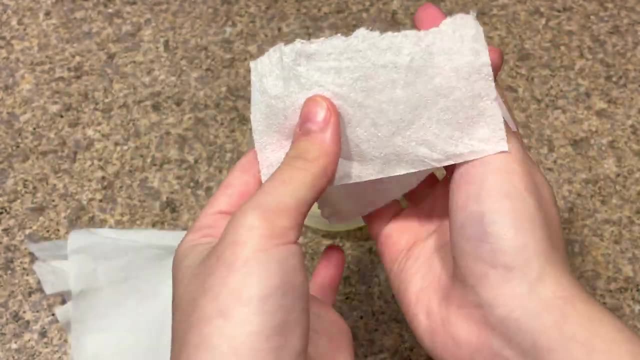 I'm going to get ripping it up just like this. I would suggest using a thinner toilet paper like this one I have, but any will do. And now for this recipe. all I'm going to do is I'm going to shred the toilet paper, just like this, And I'm going to add it into the soap. And this is going. 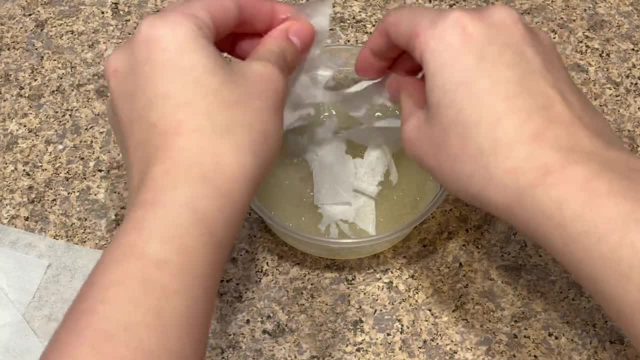 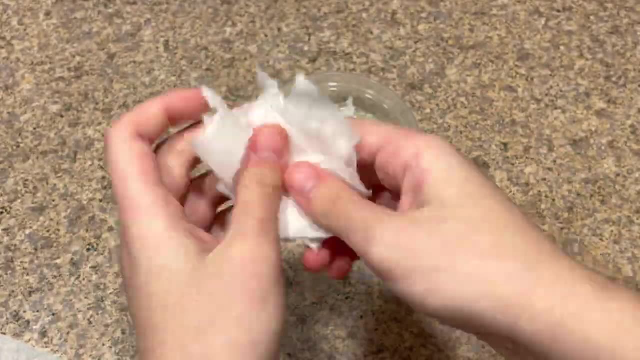 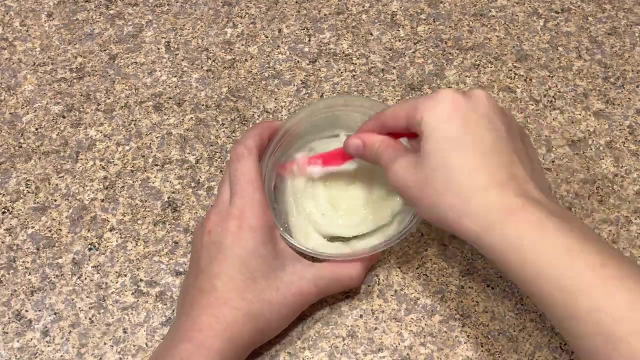 to create almost like a butter no-glue slime recipe, Kind of like a fluffy no-glue slime recipe too, And I'm just going to keep adding the toilet paper now And now I'm just going to mix this up And that's enough mixing. Now I have this really nice milky color And the toilet paper is thoroughly. 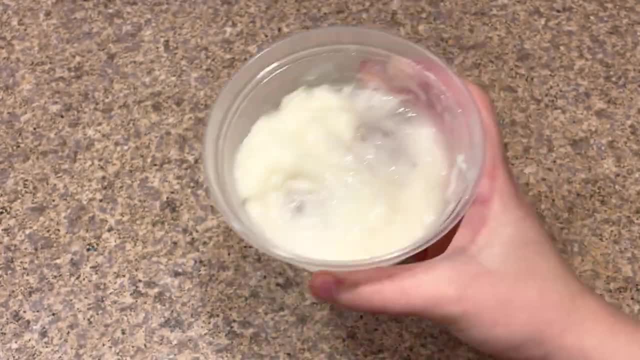 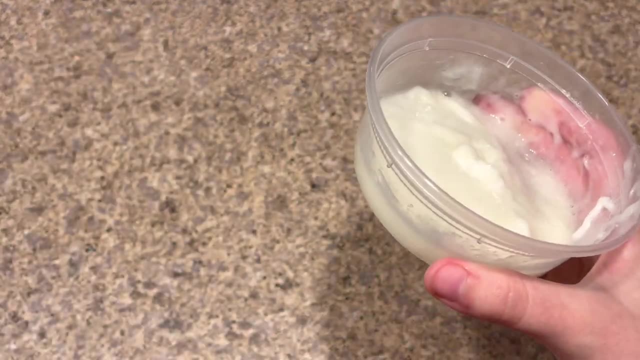 mixed in. There's a little bit of clumps in that, but that's okay. And now what I'm going to do is I'm going to put this into the refrigerator for about two to three hours. Every 30 minutes I'm going to mix it up, make sure it's working. If it needs more shampoo, I'll add more shampoo. 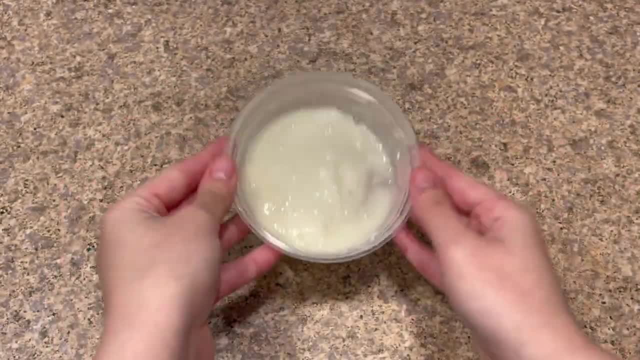 If it looks like it needs more toilet paper, add more toilet paper. So I'll see you guys in about a second. Okay, guys, So it is a few hours later. It's about two o'clock, So I'm going to mix this up. 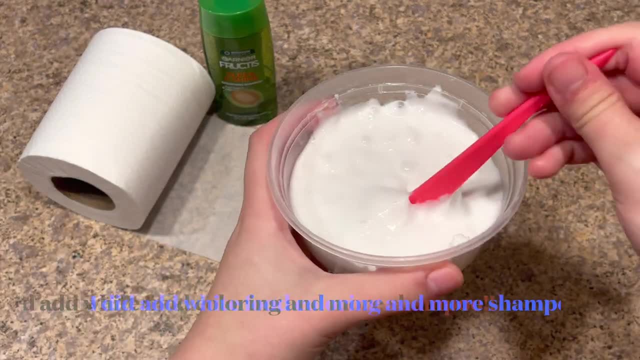 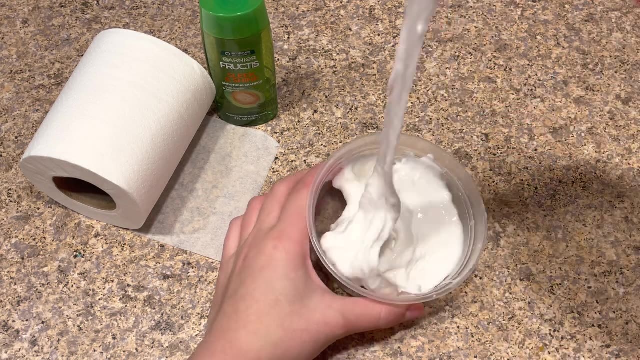 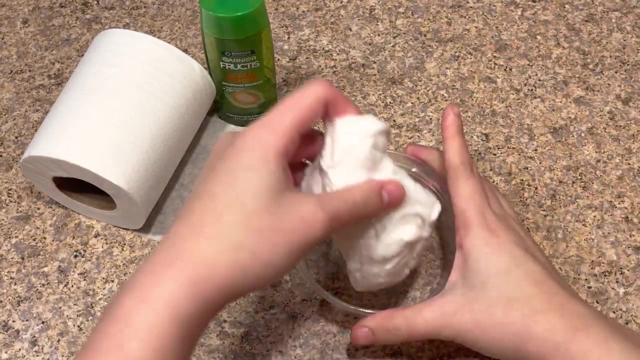 Two o'clock And here is the no-glue slime recipe. I actually added some white food coloring into here, And here it is. It looks super soapy still, But look at all the toilet paper It got mixed in really nicely. Let me see if it's sticky. Oh yeah, it's quite sticky, as you can tell, But look how. 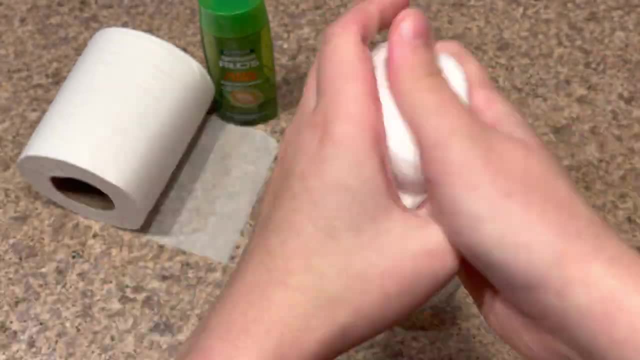 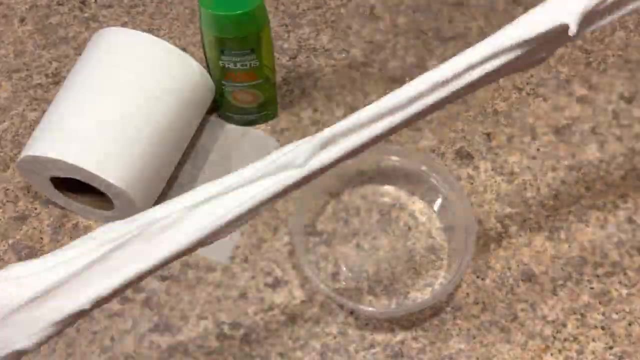 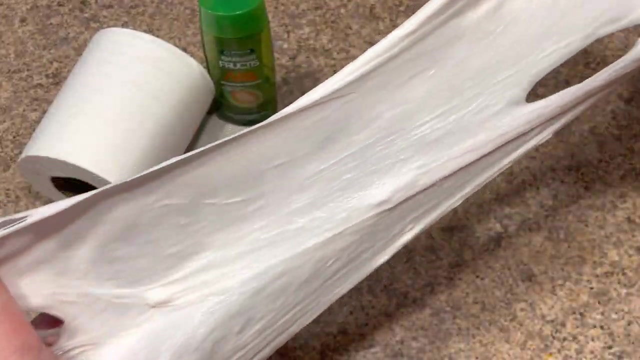 cool. this made for a no-glue slime recipe. It smells so good. It smells like the shampoo, But it's really sticky. Sorry if you hear any noises in the background- My family's really loud, But this no-glue slime recipe is really, really awesome. I'm trying to mix all the toilet paper.